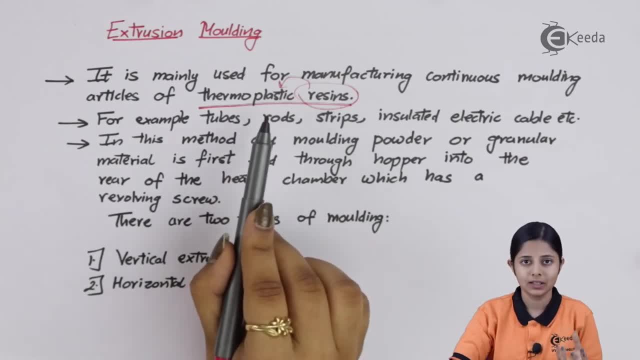 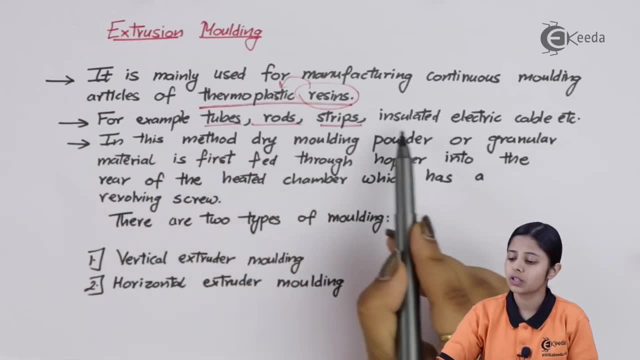 materials, Materials which have the property of thermoplasticity, and those raw materials are known as thermoplastic resins, For example, tubes, rods, strips, insulated electric cables, etc. Now, when you see the examples- all these examples are of manufacturing continuous molding articles- 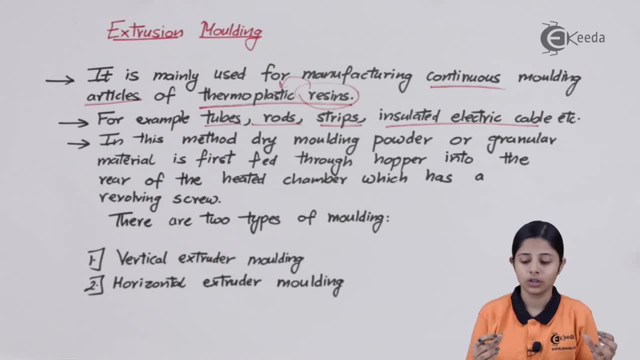 Now, these are continuous in nature. What do we mean by continuous? Now, for example, let us take a tube. A tube will start at one point and end at another point, but this is a continuous cylinder, And for such thermoplastic materials we use 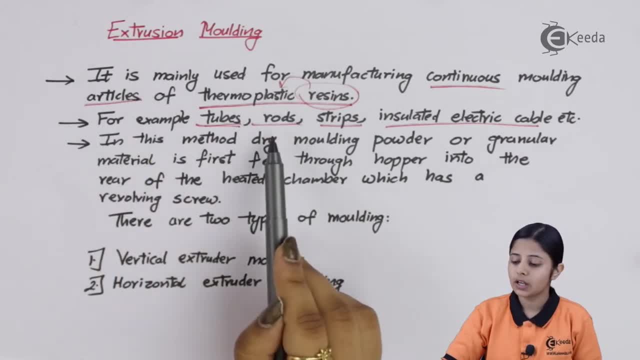 extrusion molding techniques. The other examples are rods. Again, rod is again a very long, continuous material. Strips, cable wires, cable wire insulators, all of them can be made with the help of extrusion molding In this method: dry molding powder or granular material. 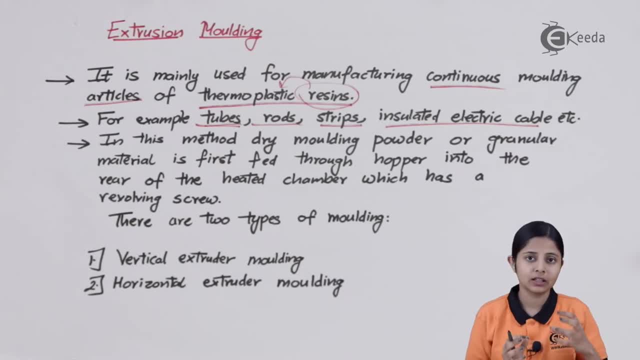 Now there are two kinds of it. You can get thermoplastics either in complete powdered form or in a form of some grains, or granular form. You can use either of them, depending on the finished goods that we need. So over here we can either use a molding powder or we can use 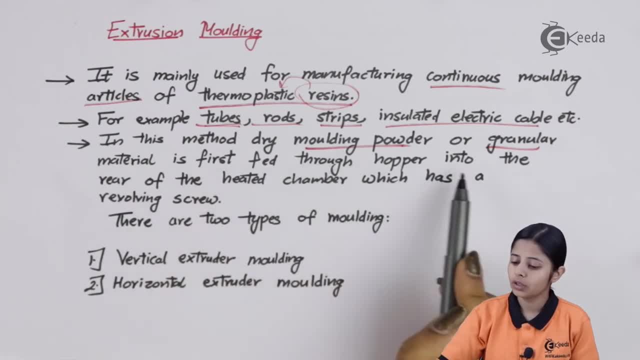 granular material. It is first fed through hopper into the rear of the heated chamber which has a revolving screw. So over here we are going to see two kinds of molds. The first is known as the vertical extruder molding and the second is known as the horizontal extruder molding- Both of them. 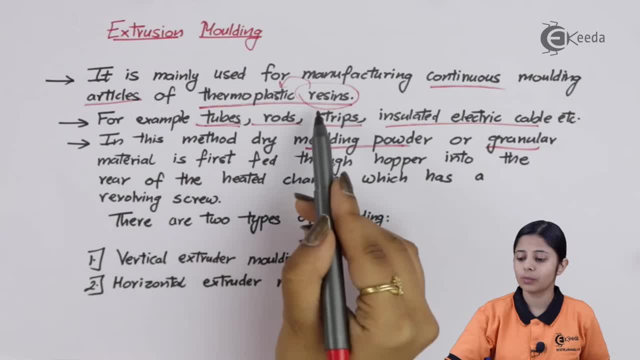 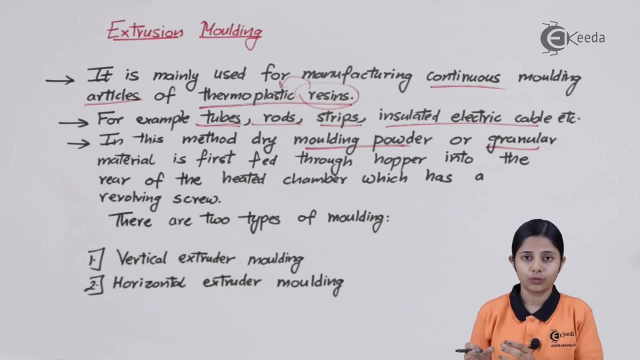 do the same thing. Both of them first take the resin that is the raw material of a thermoplastic, either in its granular form or in its powdered form, and then they make finished goods out of it. Let us see both the diagrams in detail. First, let us have a look on the vertical molding part of it. 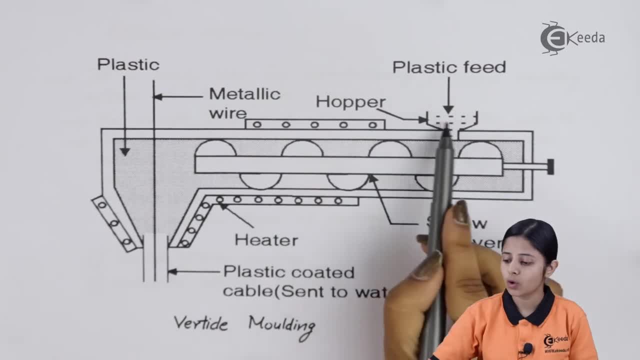 We use a hopper to just take in the resin. So over here I have this hopper and this is the plastic which is fed through the hopper. Now this plastic is fed through the hopper, So over here I have this. 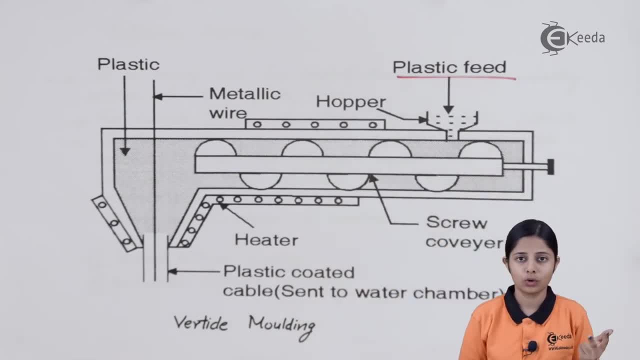 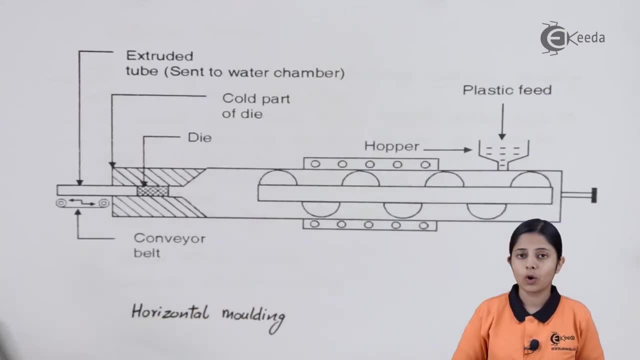 plastic fed is my resins. They can be either in the granular form or powdered form and from here it will actually go into the mold. Let us see the same for the horizontal molds. This is my horizontal mold and over here also I have a hopper, and plastic is fed through the hopper, either in. 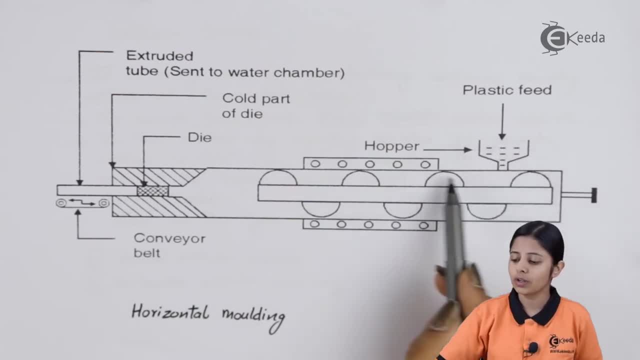 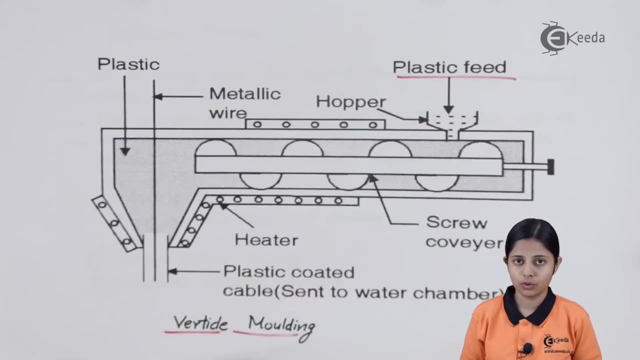 the form of granules or resins, and this plastic will flow inside this mold with the help of this hopper. This is nothing but my vertical molding. This is a part of the extrusion molding that we are doing Over here. I have an hopper. This hopper helps me to get the resin out of the hopper. 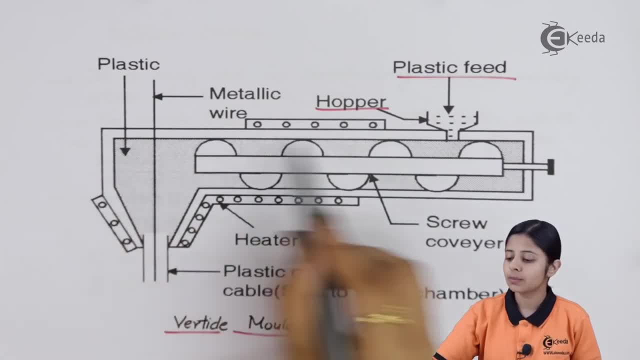 This hopper helps me to put plastic feed inside the material. This is my heated chamber over here. Now this: with the help of the hopper, we can actually find out the proportion and measure the proportions and put that kind of plastic in it and that amount of plastic in it. Over here, the 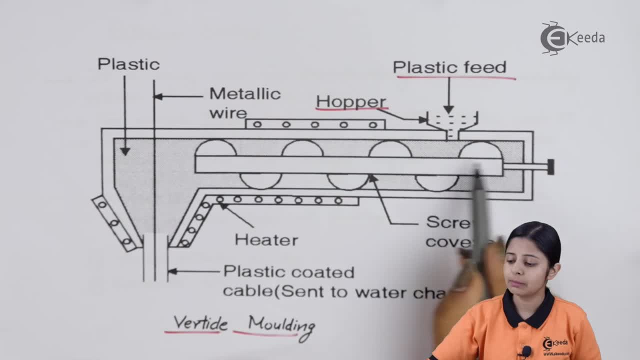 another thing which I have is a screw conveyor. This screw conveyor helps us to test the amount of plastic which is needed. If I need a plastic rod which is of this much length, I do not need to put more plastic than necessary, and that is the reason why the amount of plastic and the 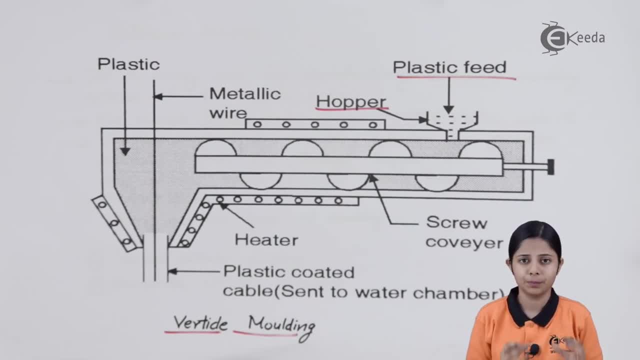 proportion of plastic which is being fed into the heated chamber is extremely important, And because of that this screw conveyor is extremely important. After that we have heaters over here. So once I have known this- the kind of plastic which gets into the hopper- I have also known 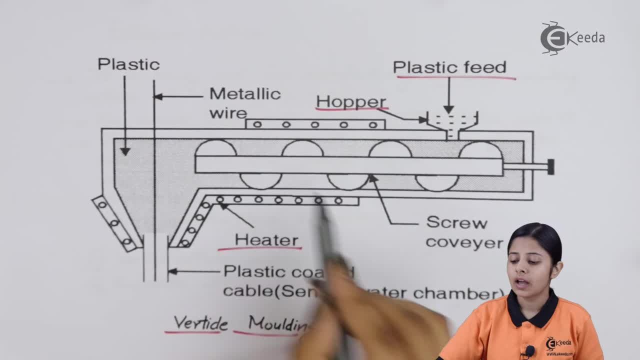 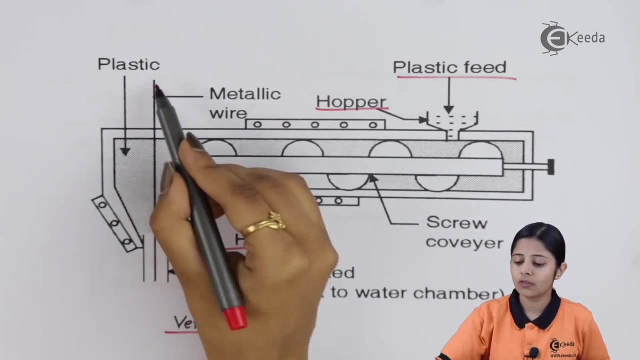 the amount of plastic which helps with the screw conveyor. I will heat that plastic over here with the help of the heaters. Over here also, I have a heater. Over here also, I have a heater. I have to make an insulating tube around it and that is the reason why I have already placed the metallic 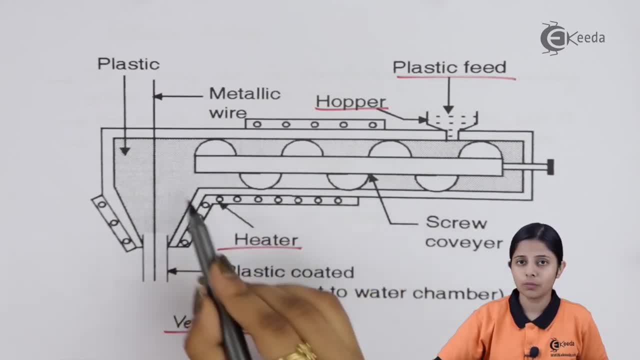 wire inside over here. Now, this heated chamber over here will heat the plastic into its liquid form and this plastic will come and wrap itself around this wire, making this wire an insulated wire. And finally, what we get is plastic coated cables sent through the water chamber. This is 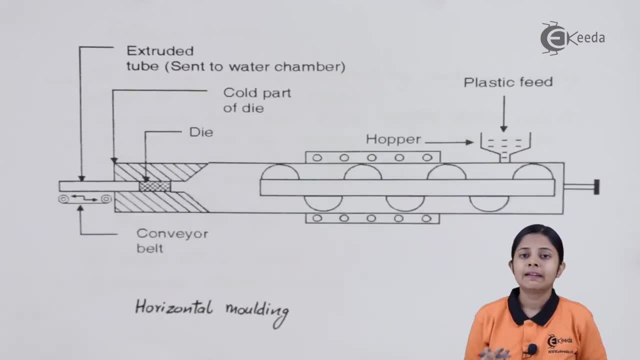 known as a water chamber, wherein we have a plastic coated cable. The exact same thing can be done with the horizontal molding. Over here we have the horizontal molding which has few parts which are similar, but few parts which are different. The similar part comes. the first one is the hopper. 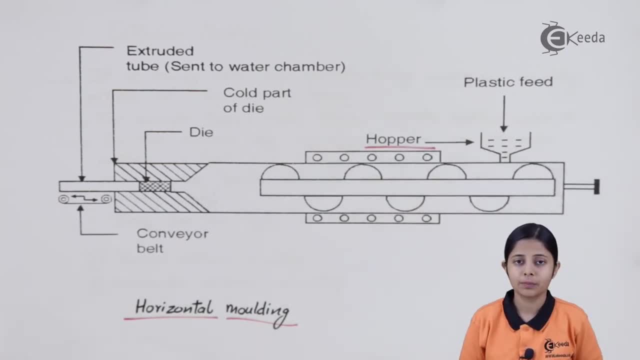 over here In the vertical molding also. we use the hopper to fed the plastic Over here also. we will feed the plastic over here inside the heated chamber with the help of a hopper. So we have plastic over here which is coming inside the heated chamber. The another thing that 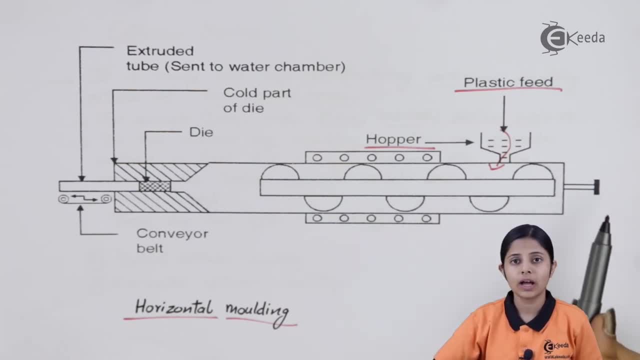 we have, which is common over here is the screw. With the help of the screw, I will know the amount inside the horizontal molding. This plastic comes over here and over here it will get heated and finally, from here I will get the wire. I have the extruded tube over here, which will then be. 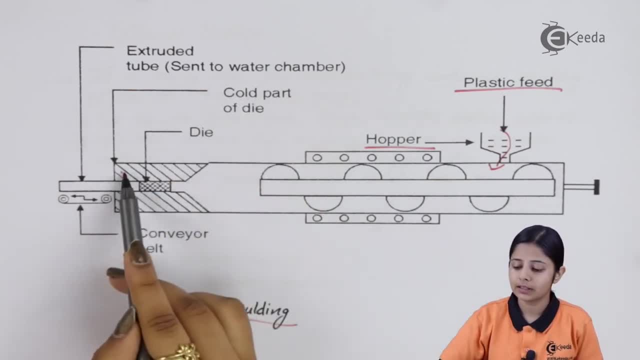 sent to the water chamber. Then I have the cold part of the die at this part and the conveyor belt over here. So this is the entire process, which can be also done with the help of the horizontal molding. When the screw is rotated, the molten material is pushed forward through the 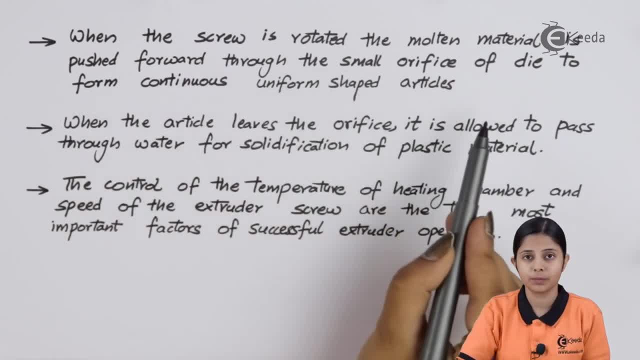 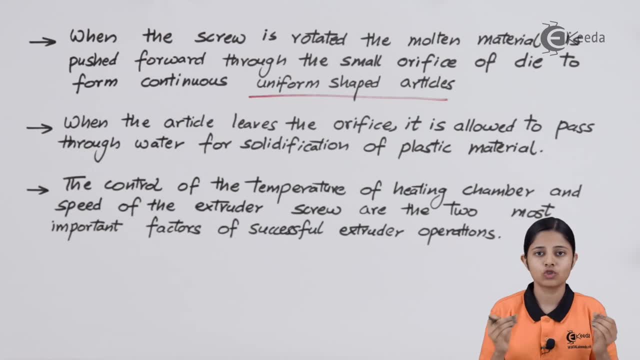 small orifice of die to form continuous uniform shaped particles. Now, these are all my continuous uniform shaped articles. Either they are rods or they are cable covers or they are long strips of plastic, But they are all continuous materials and they are not definite, small, small products of it. 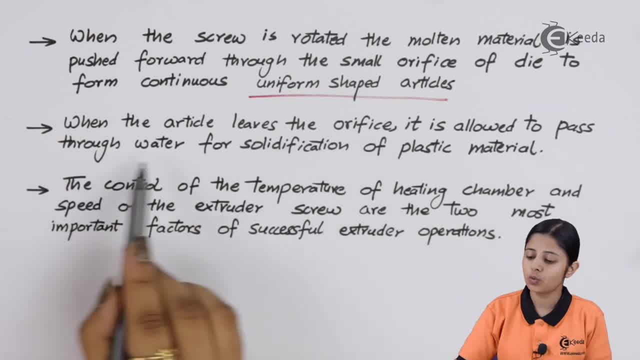 When the article leaves the orifice, it is allowed to pass through water for solidification of plastic material. Now we should understand over here that we are going through thermoplastics. Thermoplastics: on heating They become liquid, On cooling they become solid. And now, when they are becoming solid on cooling, 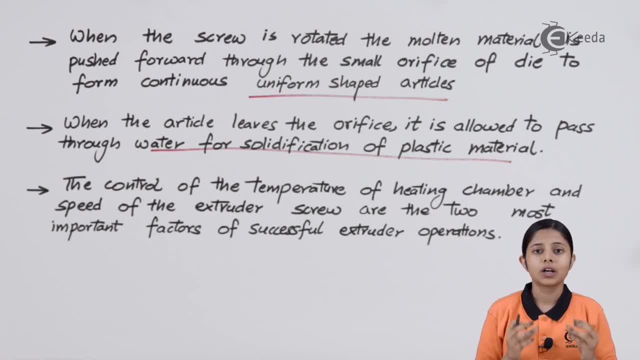 we should make sure we give them enough time for solidifying and because of that we put them into a water bath. Now, this water bath is of cold water and therefore, when these plastics come in contact with cold water, they solidify and they take the proper shape of it. The control of the temperature. 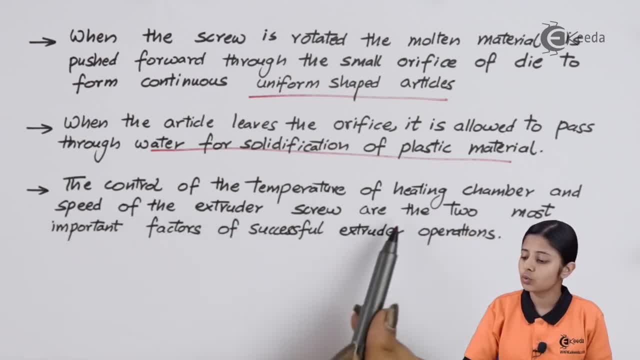 of heating chamber and the speed of the extruder screw are the two most important factors of successful extruder operations, And that's the reason why we need humor interventions only for two things: The first thing is to control the temperature of the heating chamber and the second is to control the speed of the extruder. 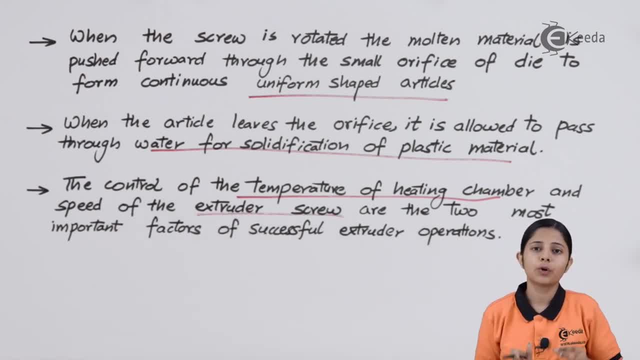 screw And once both of them are taken care of we can get proper finished products out of it. So over here in this topic we studied about the extrusion molding which happens for thermoplastics. We studied two types of moldings for it: the vertical molding and the horizontal molding. 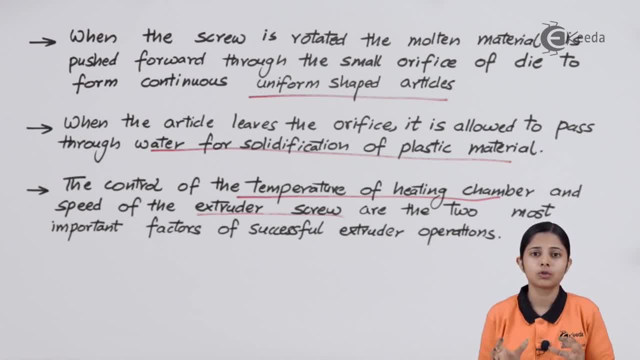 and how both of them are approximately same but a little different when it comes to the end part of the extrusion. We also studied that the finished goods obtained out of it have to be cooled with the help of a water bath. Thank you so much for watching this video. Stay tuned to eKiida and subscribe to eKiida. wwweKiidacom.